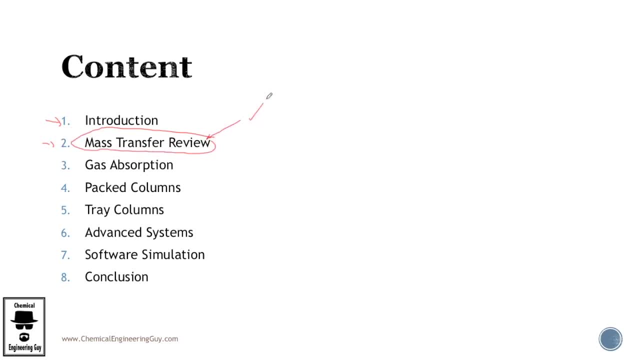 mass transfer phenomena. course, you can skip this, but actually I will definitely recommend you, just for you to remember the, the units, the variables and so on. Then we continue with gas absorption, the basics: what is gas absorption, why do we need it, what type of processes are used and some equipment. 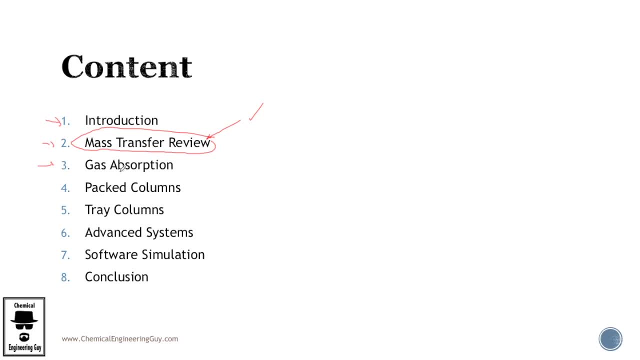 now, once we check out the gas absorption, we're going to cover these two main- I will say the most interesting part of absorption, which is packed columns and tray columns. they are, of course, inside this gas absorption part right here, but what we're going to cover here is the very dilute cases in which we have maybe 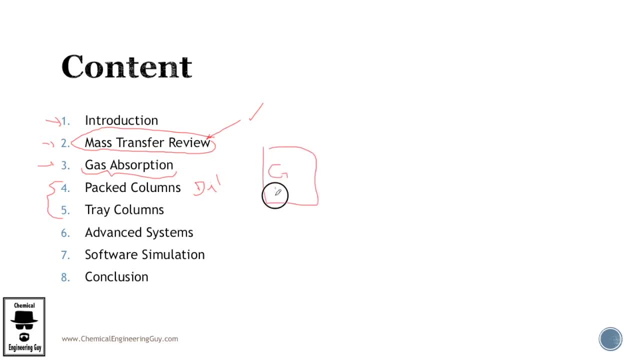 a gas with a very low concentration of, let's say, X. let's say X is a contaminant in the gas phase, and then we're going to use absorption in order to send this X to the liquid phase. so X goes to the liquid phase in very dilute amounts. let's 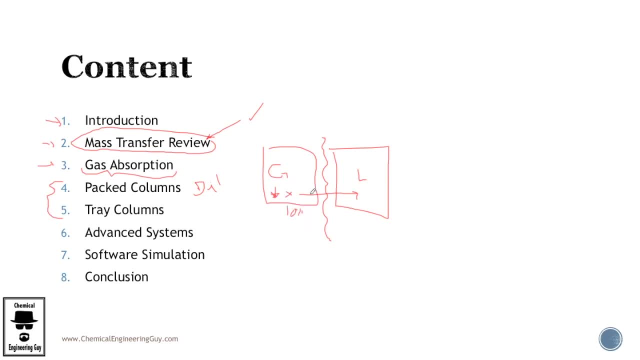 say less than 10% of X. we're going to see the path. columns, how to design them, a case study exercises the best packaging recommendations, random or order package, and so on. then we continue to tray columns. the name implies this is via trays or plates. you have the column and 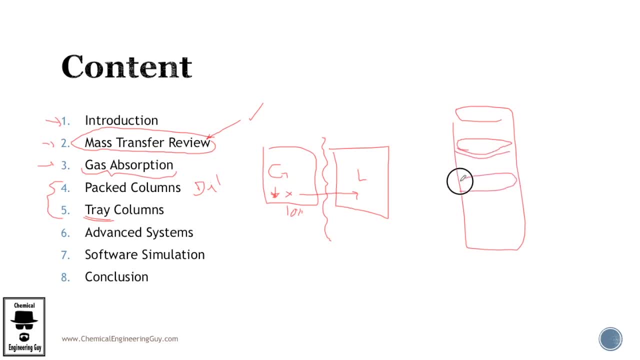 you literally, let's say physically, you separate these by trays. so what you want to do is to maximize the interaction of the gas phase, which are actually bubbles, with the liquid phase, which are going down by gravity. we see different type of trays. how do they work? advantages, disadvantages and, more importantly, we 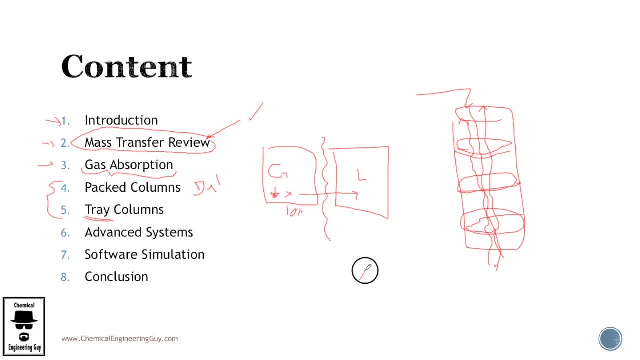 try to see which one is more convenient. each has its pros and disadvantages, pressure drops, design and so on, and I will say this is the main part of the course, or the core part: gas absorption, pad columns and tray columns. I include the theoretical concept of advanced system, which I is actually with reaction and concentrated and multi. 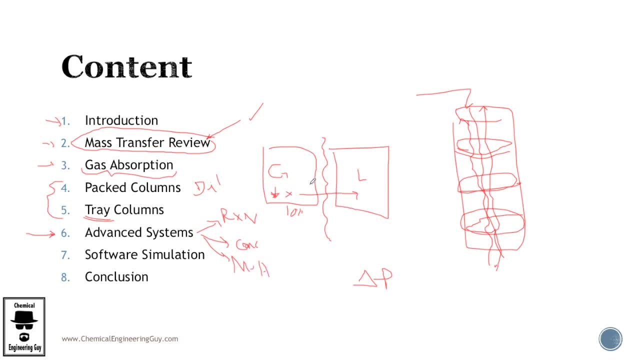 component. so, as stated before, guys, in the previous cases, we just want to learn how to interact with gas phase, the liquid phase and a very dilute X. but what will happen if you want to, or maybe you have a process in which you have X, Y and C? this is called multi component. let's say it is at low. 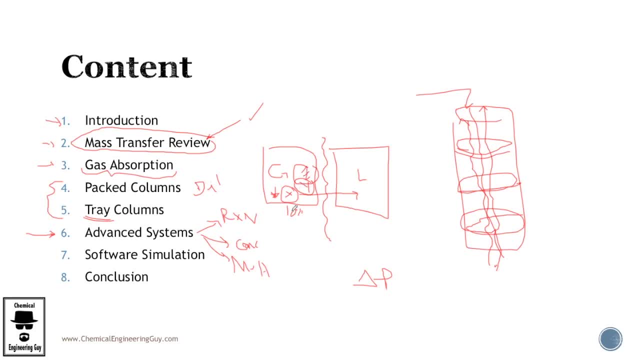 concentrations X, Y and C. this is still a multi component system. now what will happen if you have a higher concentration? maybe you just have X, but you have it at maybe 30%. well, here is mostly, mostly interesting, because the molar flow of G clearly depends on X. so that's what we're going to cover as well. 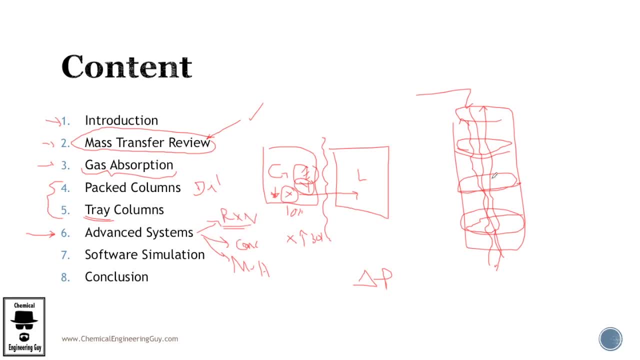 and reaction. we're going to see what happens if we have several reactions between these phases and components. this part right here, even though it seems very complex and very interesting, we're just going to cover these as a theoretical concept, maybe even propose a case for each scenario, but the idea is that you get the overall knowledge on 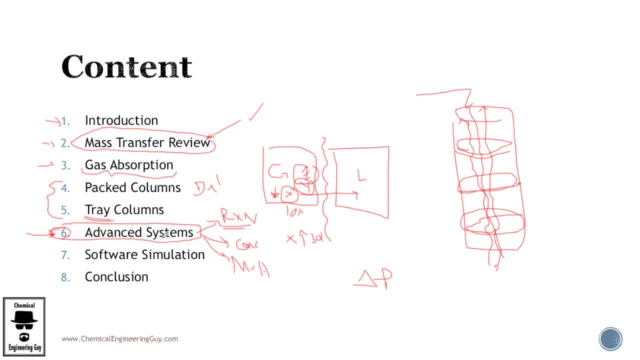 how to model these, not actually model it by hand, but we're going to do is use software simulation, actually Aspen plus. we're going to use absorption with multi-component, maybe concentrated absorption and, why not? reactions. finally, we make a conclusion on why do we need to study, how does it work? and, more interesting, I 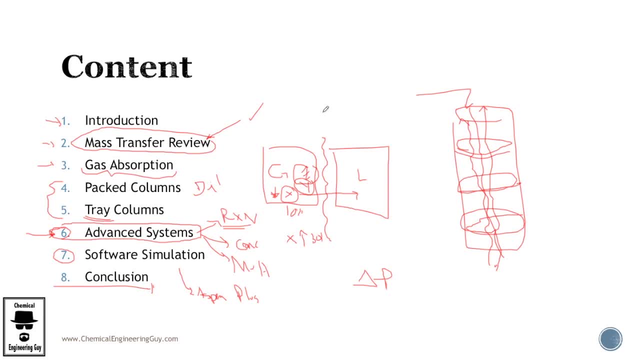 would say that absorption is one of the first units of separation processes you need to learn first. one will be flash separator, flash drum. you know that this goes as follow: you have a feed it separates gas and liquid according to their temperature and pressure conditions. but this is assumed to be one stage operation. we're going to see that in gas. 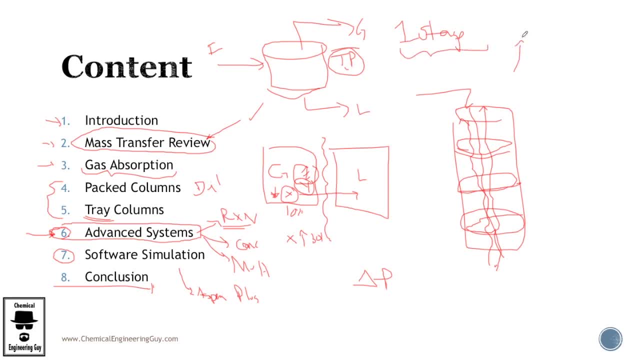 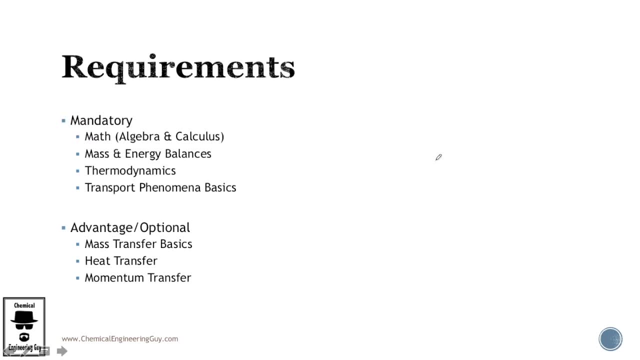 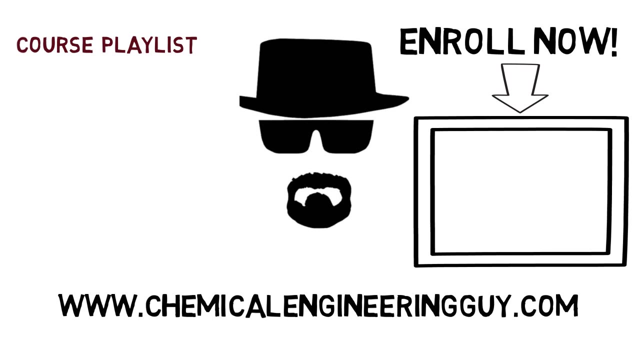 absorption we can have from one stage up to infinity stages. okay, so bear with me, let's see a little bit more on introduction you.